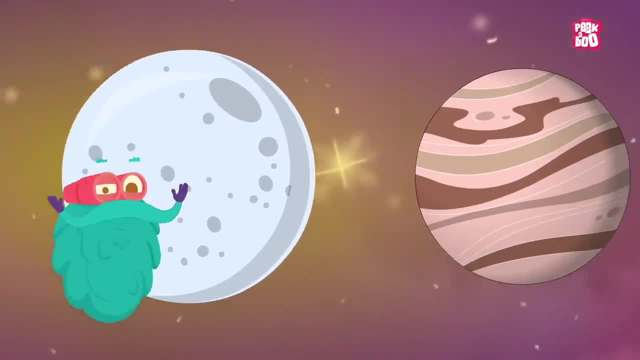 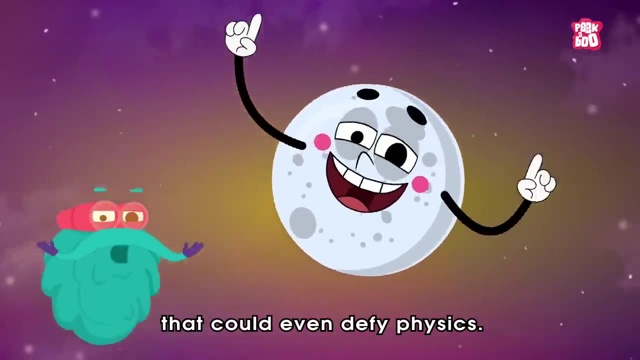 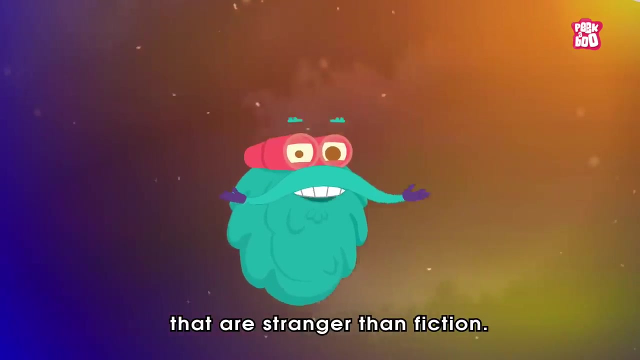 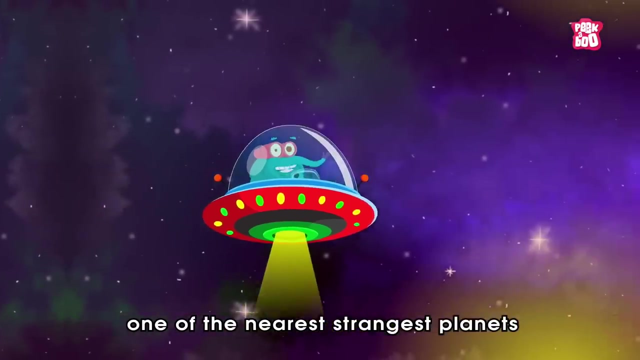 And with those kinds of numbers, there is no surprise that few of these planets will exhibit a strange phenomenon that could even defy physics. So let us explore 5 such worlds that are stranger than fiction. First, let's go to one of the nearest strangest planets. 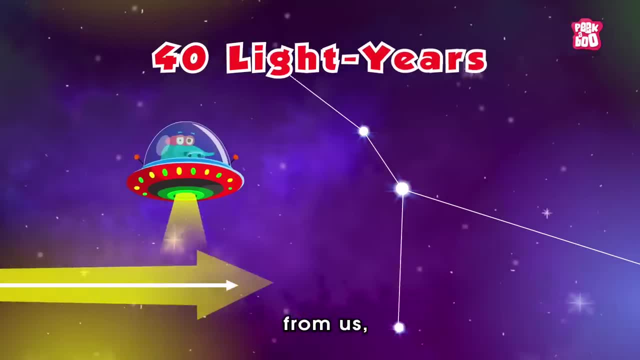 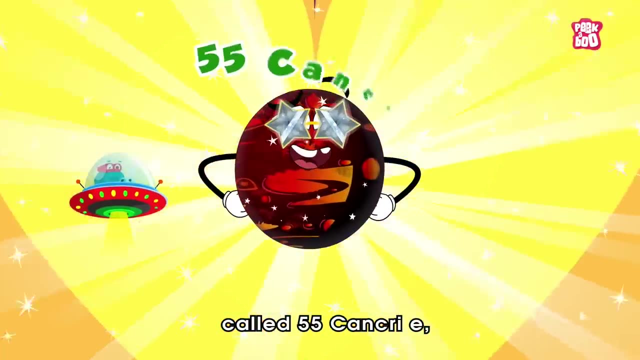 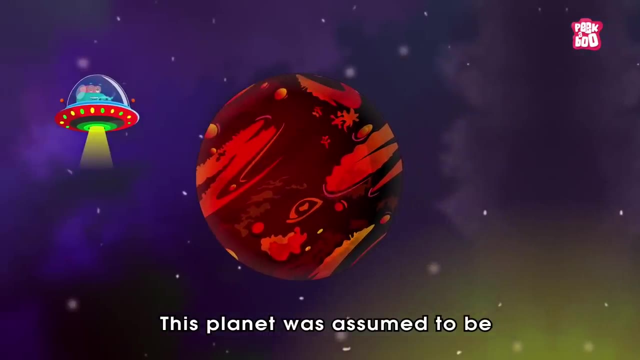 located around 40 light years away In the Cancer Constellation To see a world made of diamonds called 55 Canceri E, also known as Janssen. This planet was assumed to be so abundant in carbon that, due to the immense pressure and hot temperature, 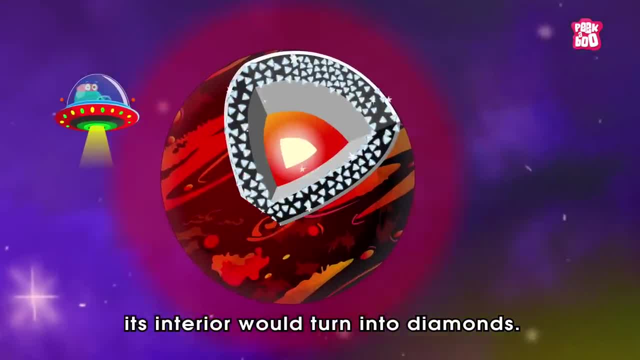 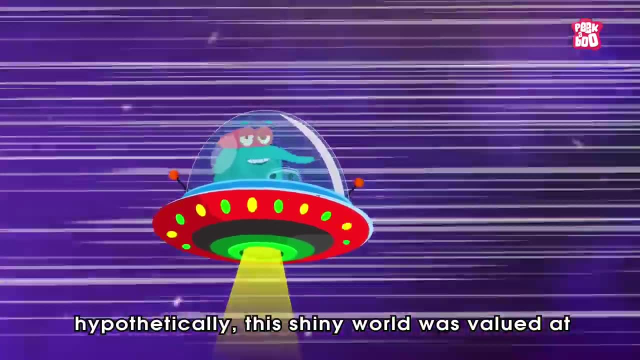 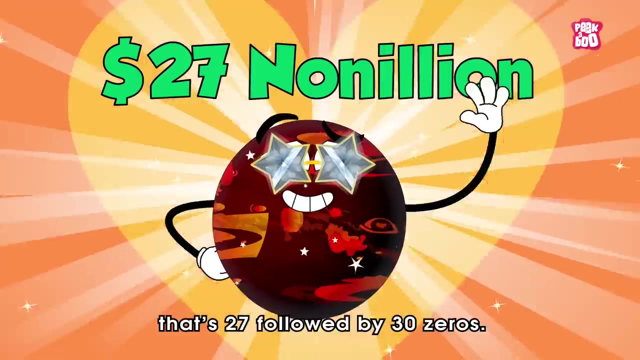 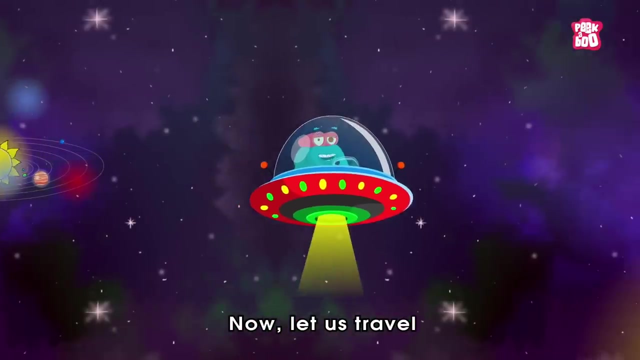 its interior would turn into diamonds, Though there is still a lot we need to know about it. hypothetically, this shiny world was valued at 27 nonillion dollars. That's 27, followed by 30 zeros. Now let us travel nearly 48 light years away from Earth. 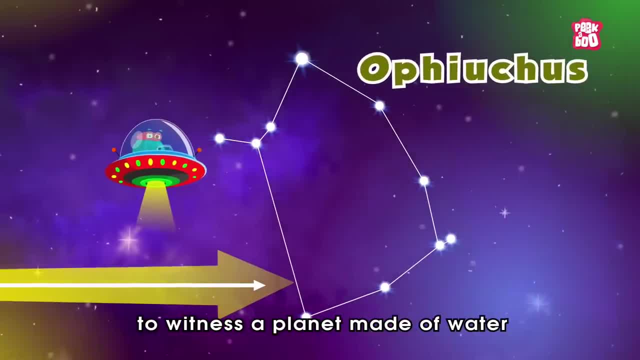 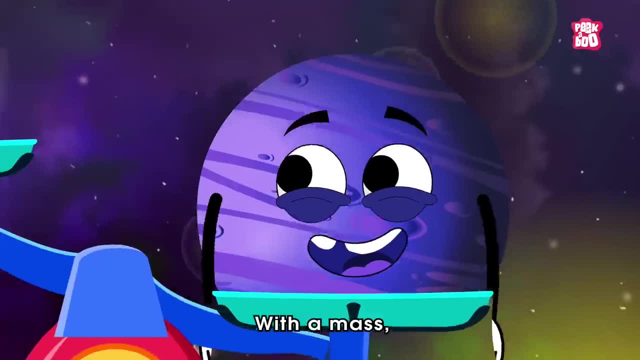 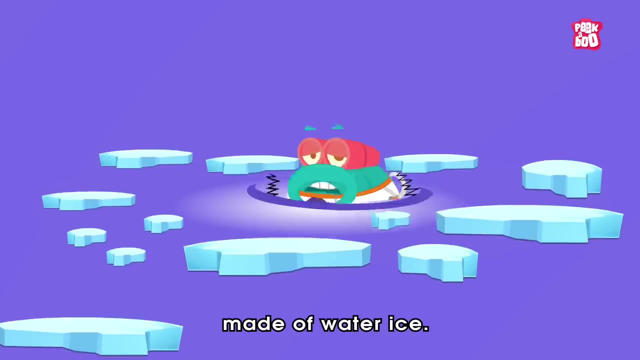 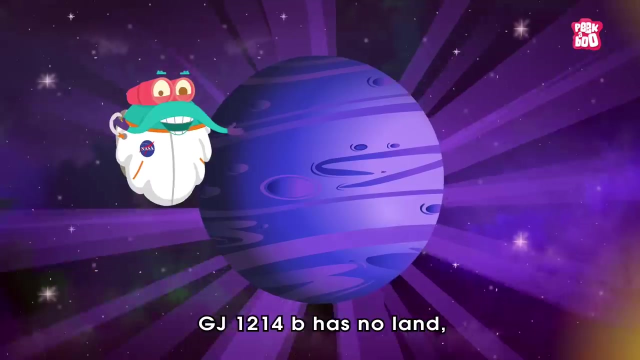 in the constellation Ophiuchus to witness a planet made of water called GJ 1214b. With a mass about 6 times that of Earth. its interior is likely mostly made of water ice, So many scientists assume that GJ 1214b has no land. 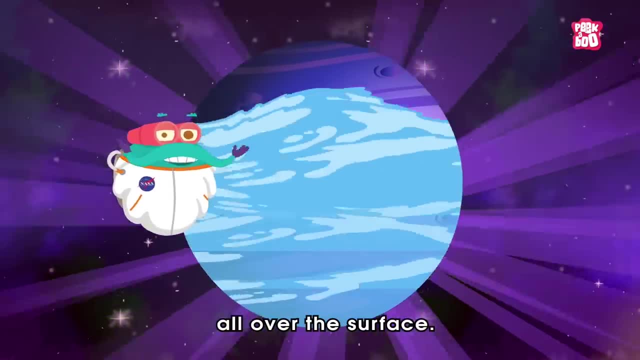 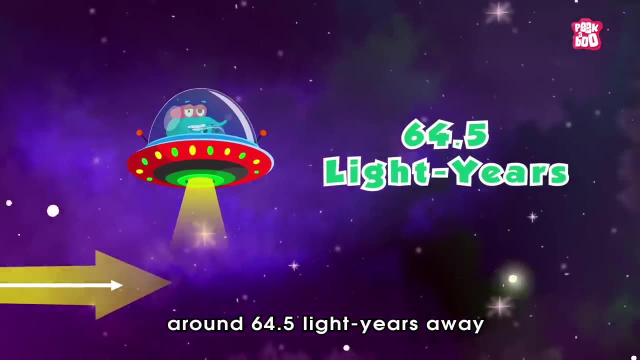 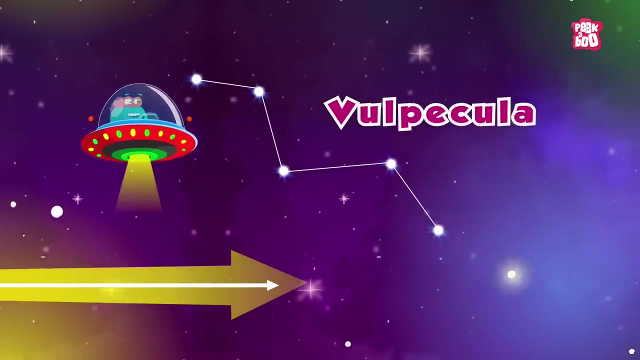 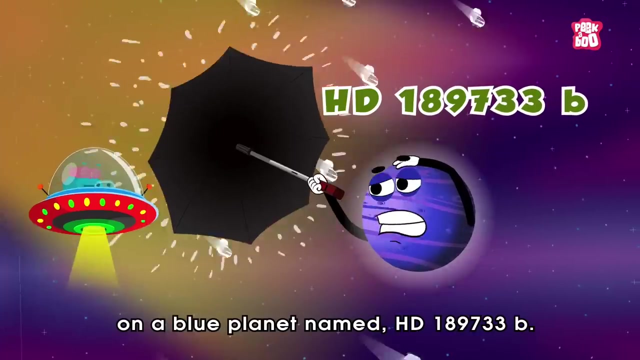 but only oceans that stretch all over the surface. Now let's go a bit further, around 64.5 light years away from our solar system In the constellation of Vulpecula, to witness the reign of terror on a blue planet named HD 189733b. 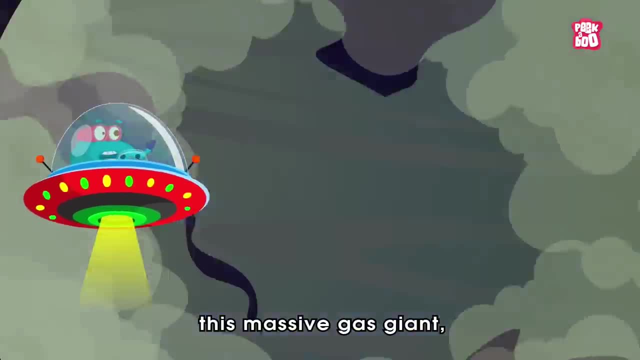 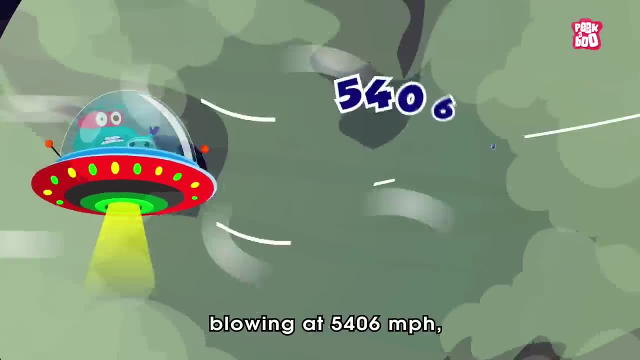 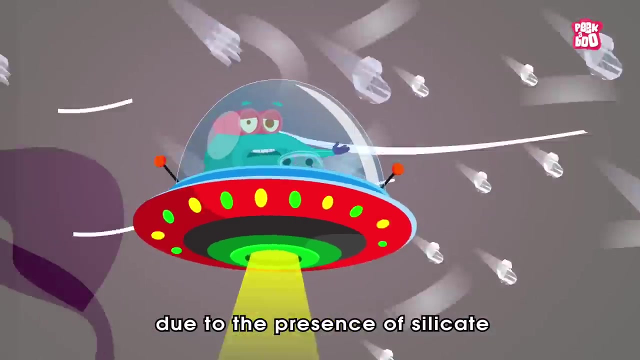 If you had the misfortune to visit this massive gas giant, you'd be spun furiously by winds blowing at 5406 miles per hour and you'd be cut into shreds by glass rain due to the presence of silicate in its atmosphere.